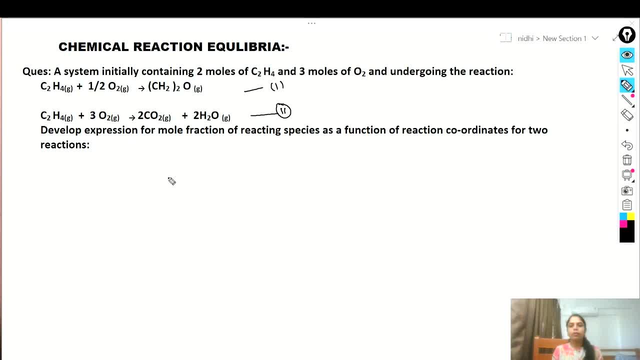 for mole fraction of reacting species as a function of reaction coordinates for two reactions. So in the previous question which we had solved in that we need to develop expression for individual reactions, Here we need to develop the combined expression for both the reaction. So first, what we do, we just write down species. 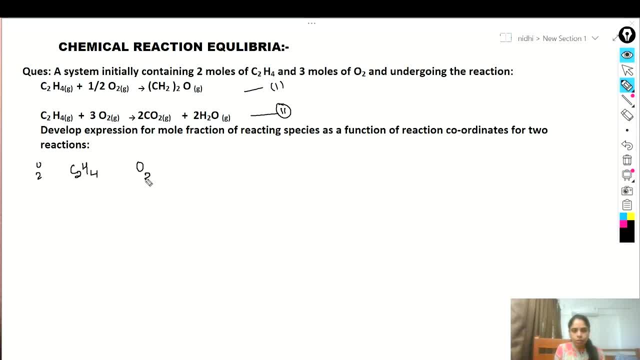 So we have number of species, C2H4, then oxygen, and we have CH2O, then we have CO2, which is not common, right H2.. So these are the two reactions. So we have C2H4 plus 3 O2 gives 2 CO2 plus 3 H2O. So 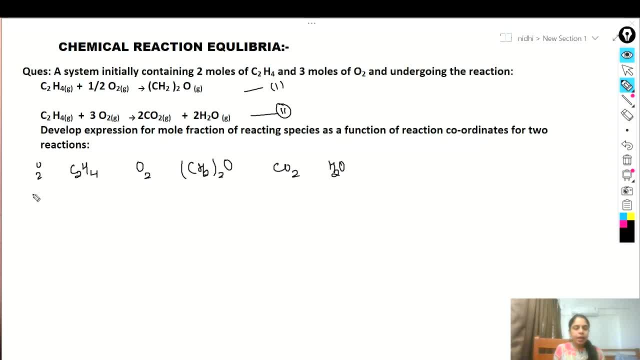 these are the two reactions. So in the previous question which we had solved in that, we need to develop the combined expression for mole fraction of reaction. So this is your second reaction. So this is your second reaction. So these are the different species which we have Now. J here it denotes the reactions. So reaction 1, we have reaction 1 and reaction 2.. 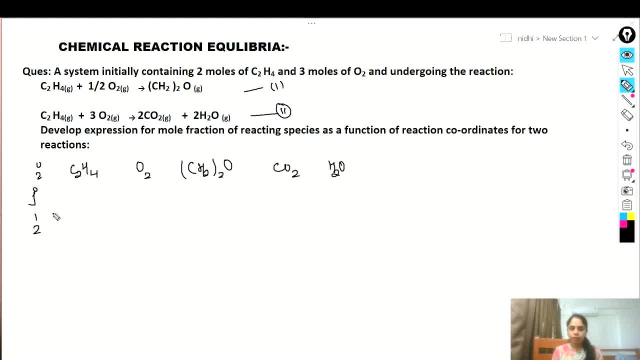 And then we need to write down the stoichiometric coefficient of reaction, stoichiometric coefficients of species in reaction 1 and reaction 2.. So in reaction 1 it is minus 1, C2H4 minus half, or you can write 0.5, then this is positive. So this is positive. So in reaction 2 we have C2H4. 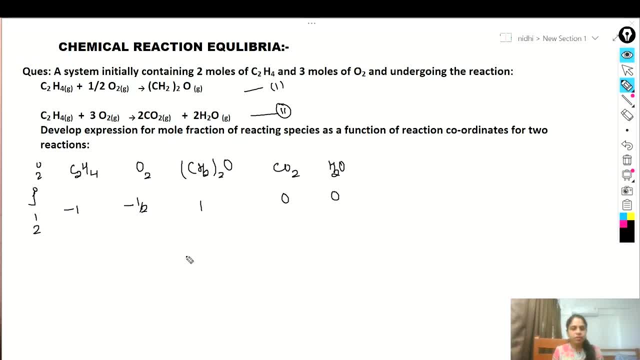 so 1. these two are not present in the first reaction. in the second reaction, c2h4, the stoichiometric coefficient is minus 1, o2 minus 3. this is not there and this is my plus 2 and this is also plus 2. now we need to write down this overall stoichiometric coefficient for reaction. 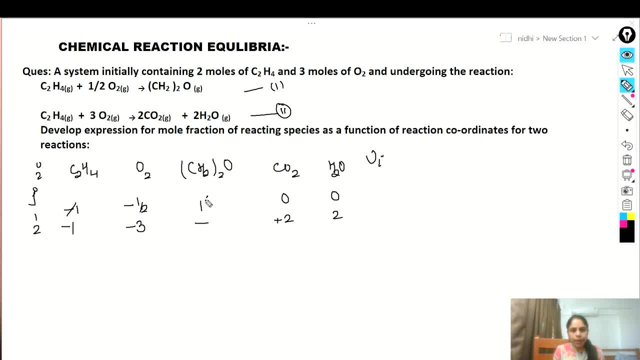 1 and reaction 2. so for reaction 1, 1, 1 cancelled. so it is minus half, or you can say minus 0.5 here, plus 2 plus minus 4, so this is 0. okay, and the total given total number of moles given total. 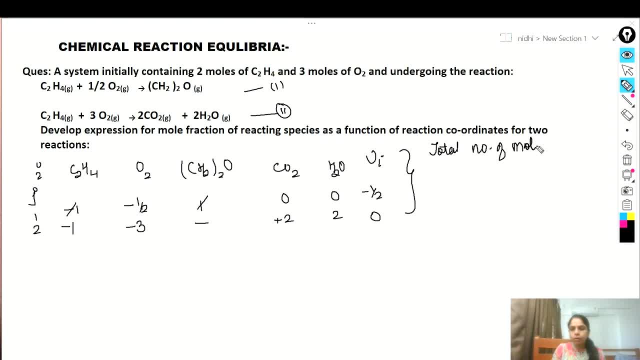 number of moles. so which is n, o and naught which is 2 plus 2. initially 2 and 3, so total 2 plus 3 is 5. okay, so now write down the expression for the first ones: y, c2h4. 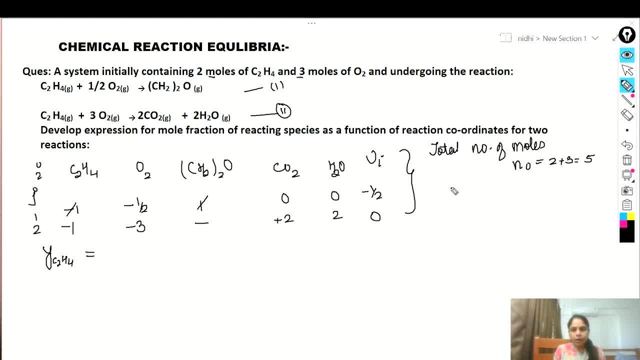 gas phase. So we know that the formula we have formula is Ni0 plus mu I epsilon upon N0, which is the overall total number of moles. mu is overall stoichiometric coefficient and epsilon is extent of reaction. Here we have two reactions so we need to write two: extent of. 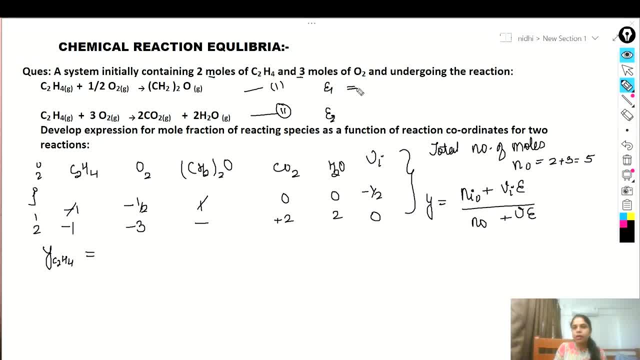 reactions. for this is for the epsilon, 1 is for the extent of reaction, for extent of reaction for reaction 1, and this is for the reaction 2.. So now write down. so we have: initial number of moles of C2H4 is 2, then stoichiometric coefficient of reaction: 1 is minus 1, so minus. 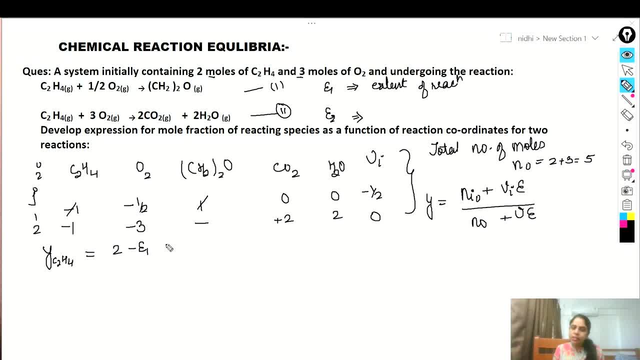 epsilon 1, fine second. for the second one is 0.. For the second reaction is also minus 1 to minus. epsilon 2 divided by total number of moles are 5, so 5 plus for the first reaction it is minus 0.5 epsilon 1, then 0 epsilon 2. 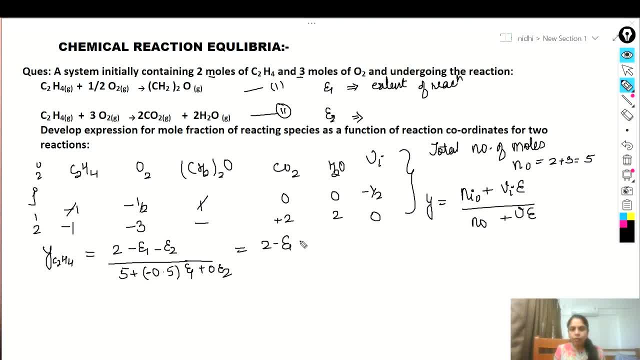 so this will be equal to 2 minus epsilon 1 minus epsilon 2, divided by 5 minus 0.5 epsilon 1.. So this is the expression for C2H4.. Okay, mole fraction of C2H4. now for the second one, Y02. so initial number of moles of oxygen. 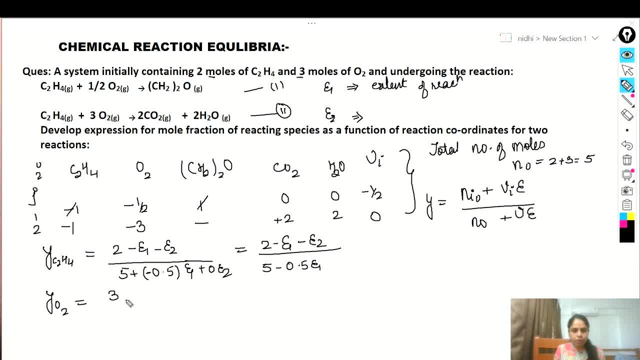 is 3, fine, stoichiometric coefficient is minus 0.5, epsilon 1. and for the second reaction, minus 3, epsilon 2. and denominator: we know that it remains same, so it remain same, fine. Now, third one is YCH2.. So initial number of moles are. there is no initial number of moles, so 0 plus stoichiometric. 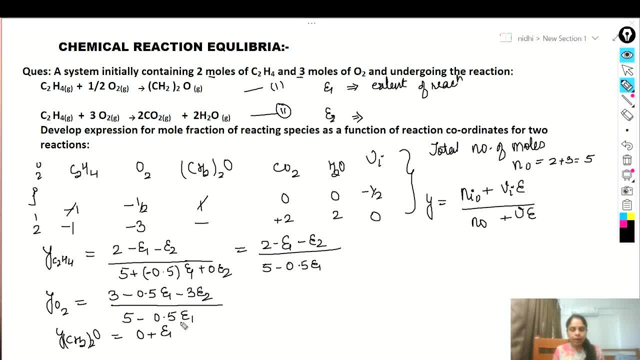 coefficient is 1, so plus epsilon 1, and in the second reaction it is not there, so 0 epsilon 2, and denominator is remain same for everyone. so this will be equal to epsilon 1 upon 5 minus 0.5 epsilon 1..